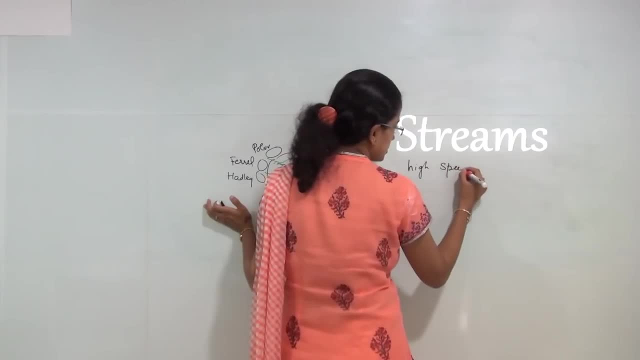 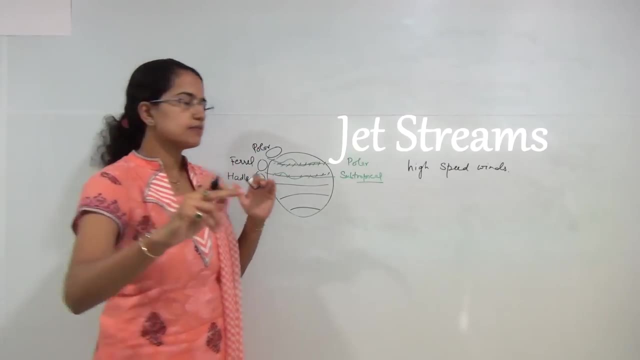 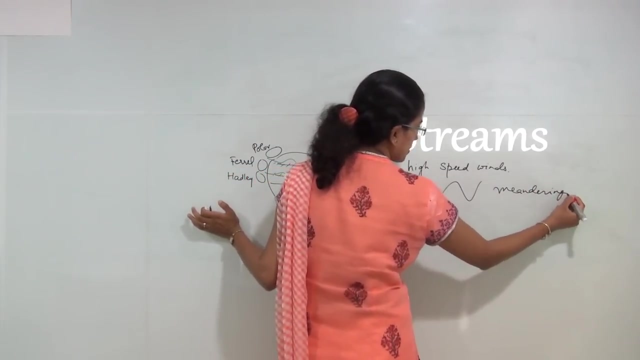 So you have high speed winds. these blow not in a regular fashion, So they can. I can say they blow in a meandering fashion. So they have meandering bands that are formed. They are irregular in nature. So they are irregular in nature. 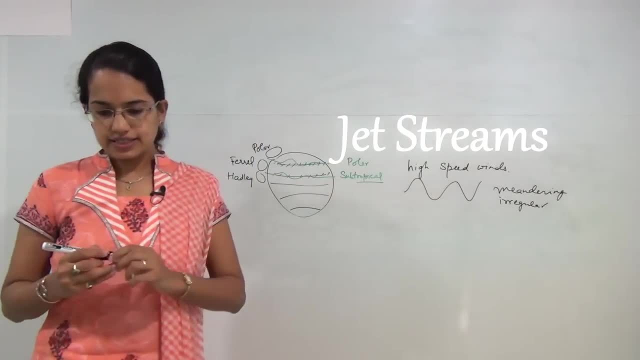 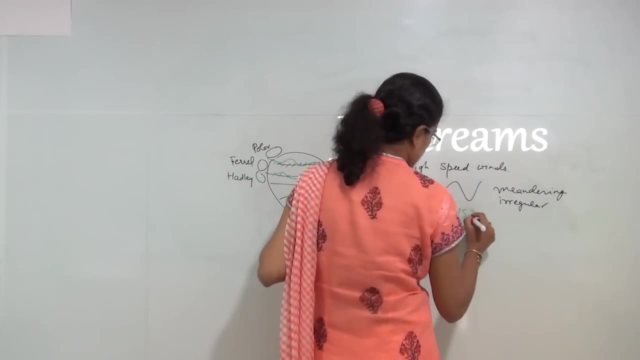 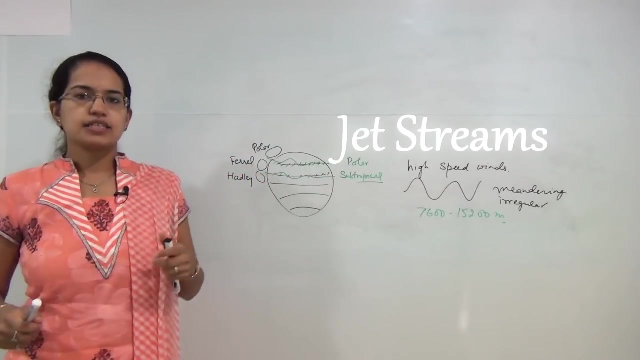 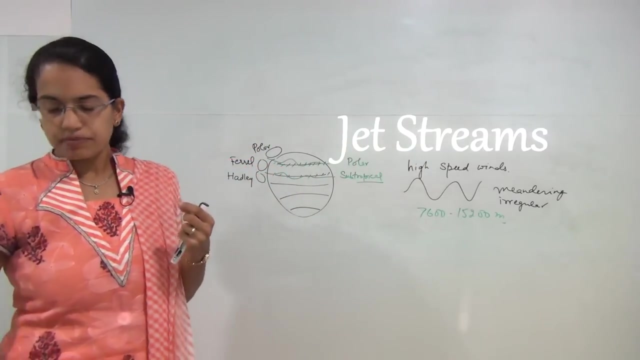 Again, I can say they are concentrated to specific areas. They are found at about 7000 to 15000 meters above the earth surface and the speed is around 250 to 550 kilometers per hour. So these are some of the common characteristics, or I could say major characteristics, of jet. 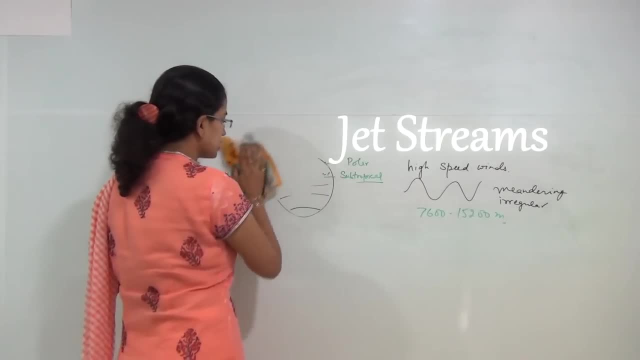 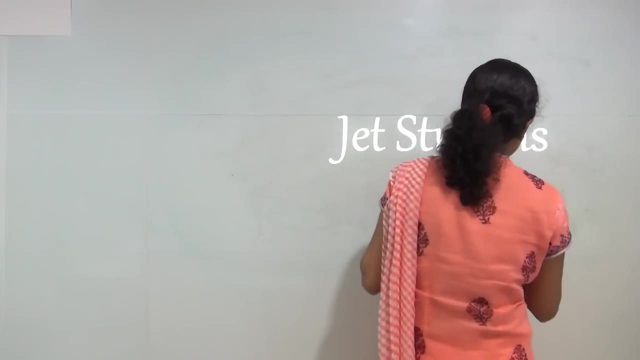 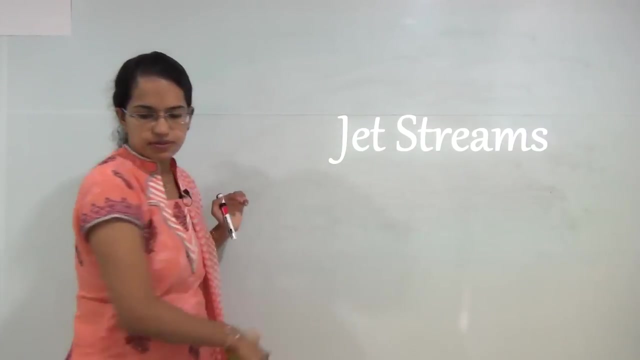 streams. Now, because of jet streams, there is a strong turbulence Because of the wind, shear and the aircrafts that are moving into the upper troposphere need to take care of the passengers and, because of the safety issues, they need to know the regions of jet streams. 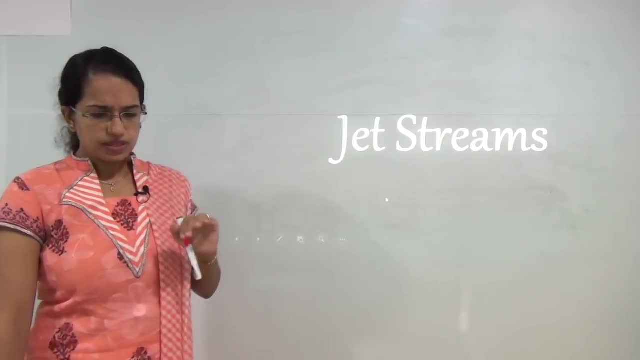 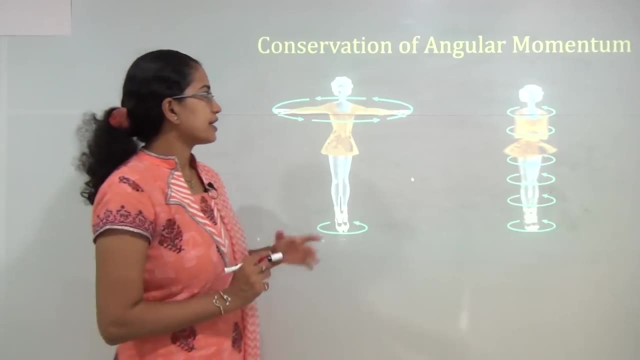 So they avoid the areas of jet streams. Again, once you know the pattern of jet streams, you can plan out the route information based on that. Now, to understand the jet streams and the intensity of the jet stream, you have to understand the jet stream. 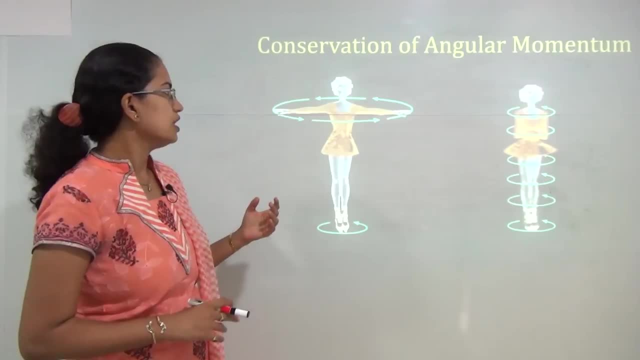 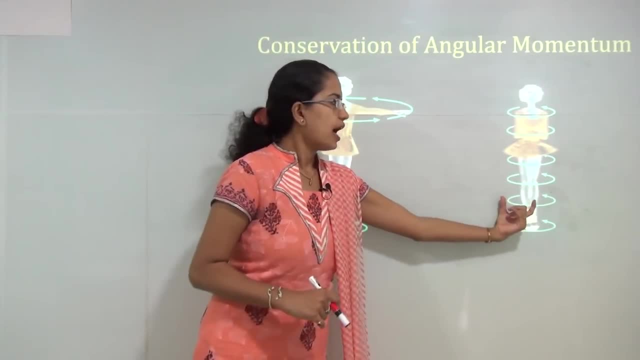 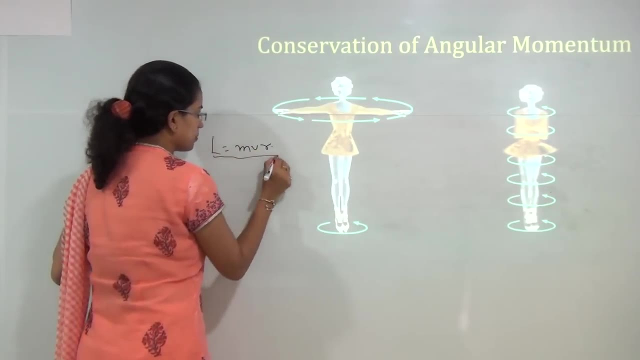 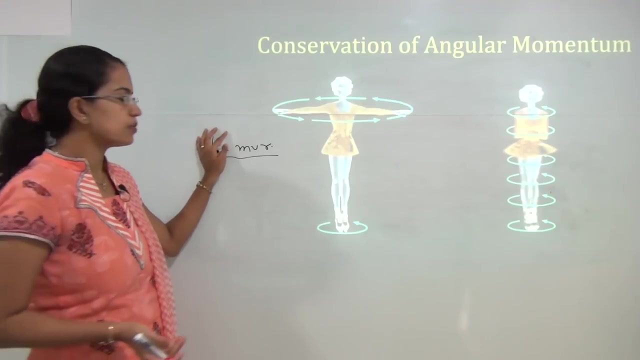 So you have the 2 images here and what we are trying to explain is the conservation of angular momentum. So when I say angular momentum is a product of mass, velocity and radius, If I want to conserve the angular momentum, since the mass of both the girls here are same- 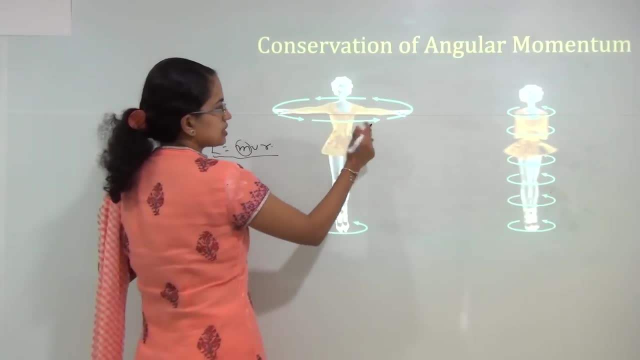 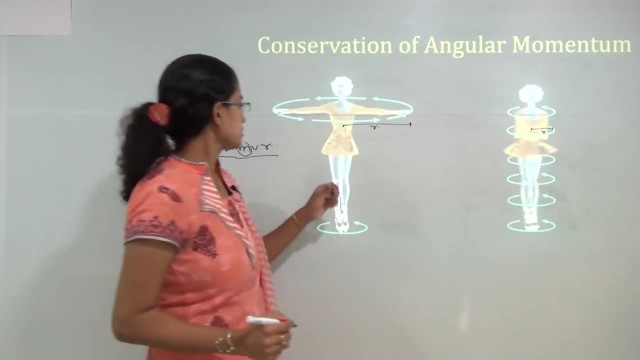 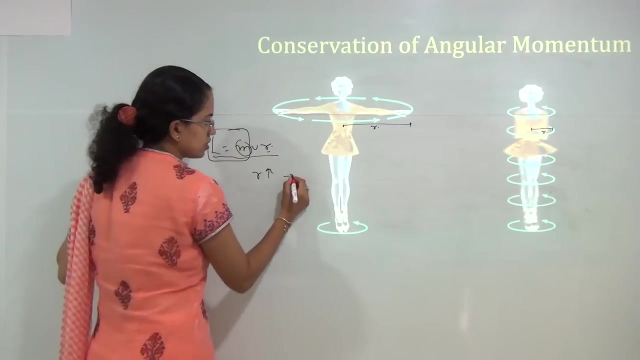 in this case, when they are spinning around. in this case, the radius is more and in this case, since the hands are close, the radius is less. so, since I want to conserve this quantity, what would happen if r is more? velocity would be less or the speed of the girl would be less. 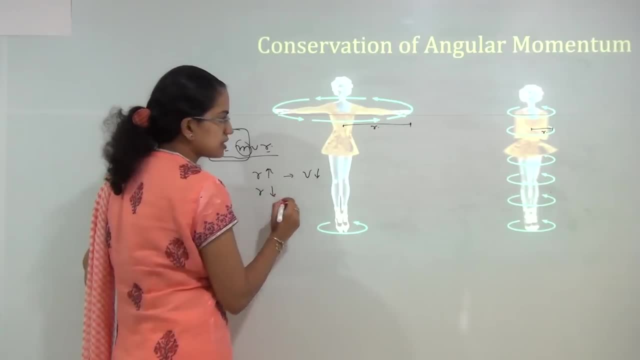 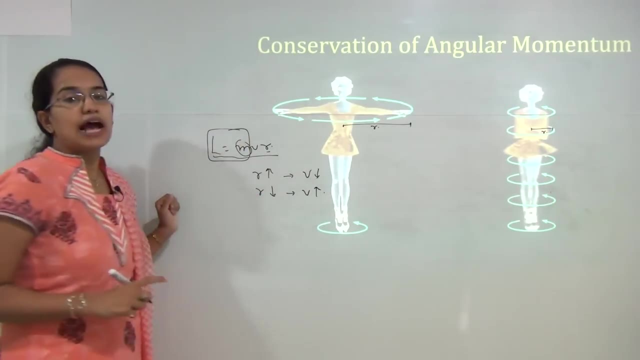 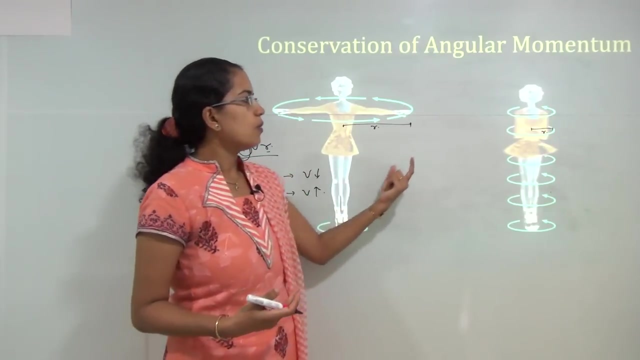 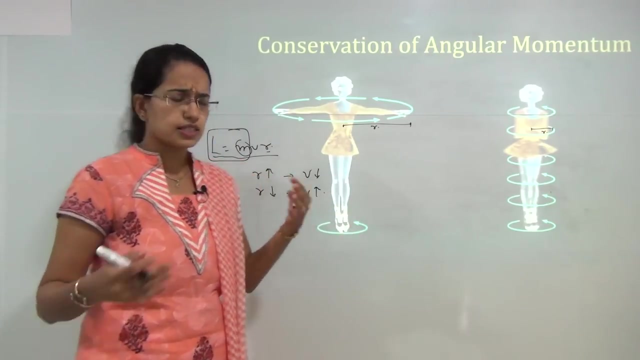 but, however, in the second case, when the radius decreases, when the hands are shrink closer, the radius decreases. as a result, the velocity increases, and similarly happens with the jet stream. So when we understand the formation of jet streams, we will see how the radius of the jet stream decreases and once the radius decreases, the velocity of the jet stream increases. 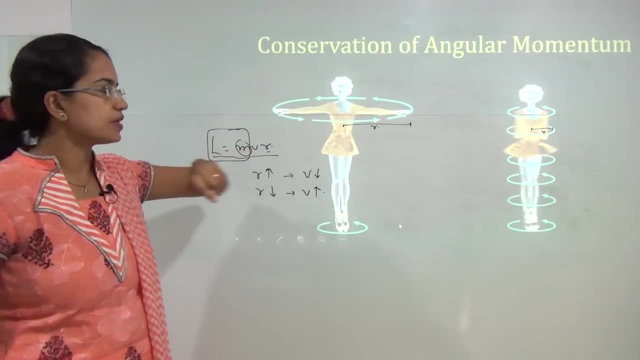 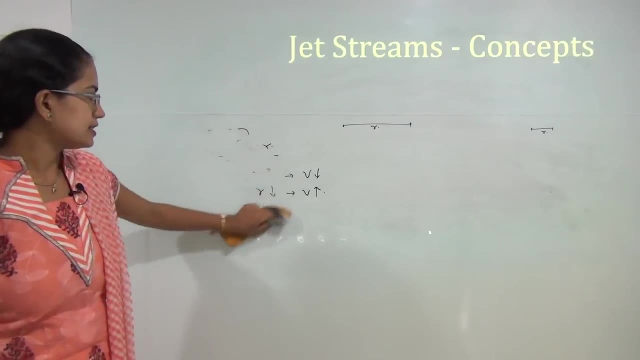 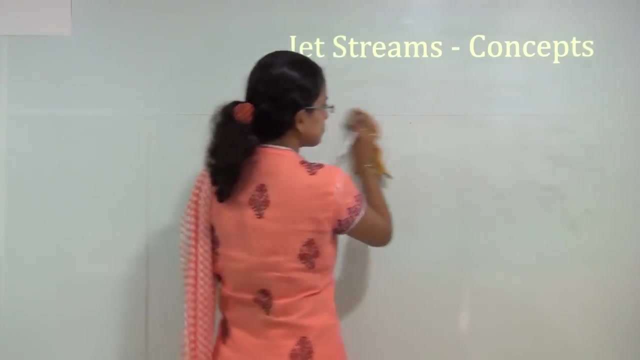 So therefore, understanding conservation of angular momentum is very important to understand the jet streams. Now jet streams formation, when we talk about, I can say we will understand the formation in two basic criteria: first is the polar and the subtropical jet stream and the second is the tropical jet streams. Now the formation of the polar and the subtropical jet streams would be more or less the similar. so I can say polar, subtropical and mid latitude jet streams would have similar kind of formation technique and you would have a separate formation mechanism for tropical easterly jet streams. 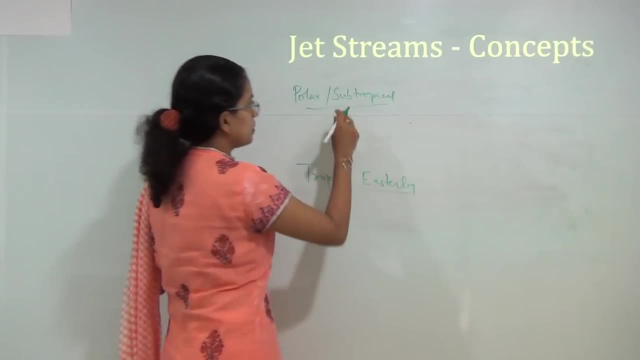 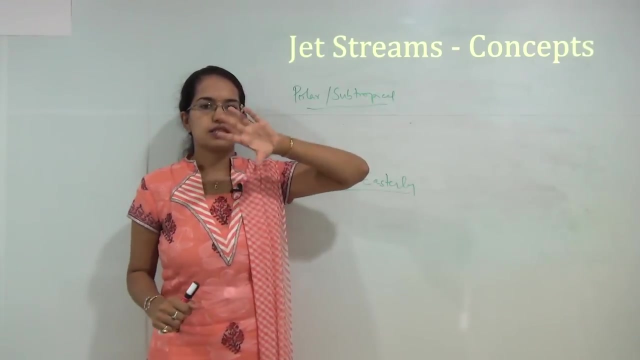 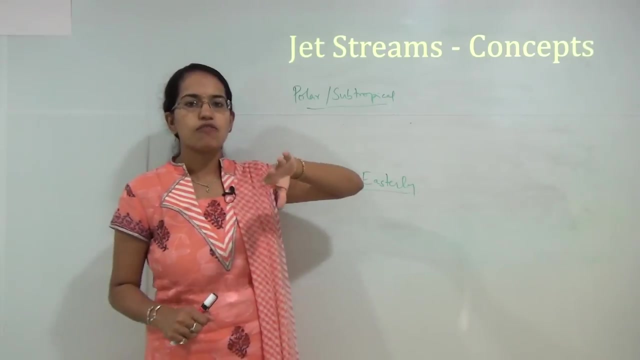 So we will understand the formation of the jet stream Now, the polar or the subtropical jet streams. as I said, in the north the polar jet stream is around the regions of North America, Europe and northern parts of Asia. in the south, they are around the regions of the polar jet stream is around the region of antartica. 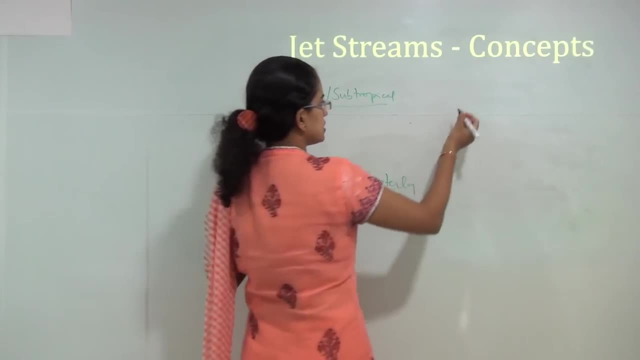 Now, these both the jet streams, follow the three cell model. so, as I mentioned, they are located on the boundaries of the three cell model. So you would have one jet stream, the subtropical jet stream, and the subtropical jet streams would be in the north. 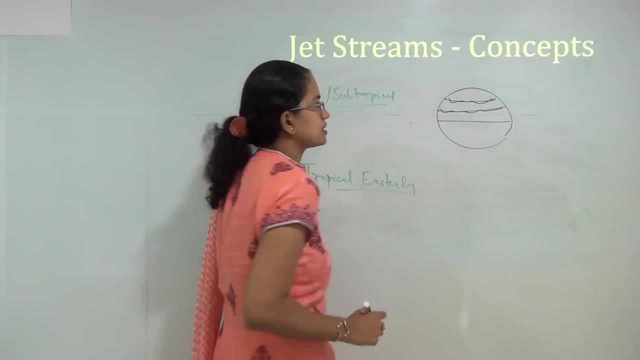 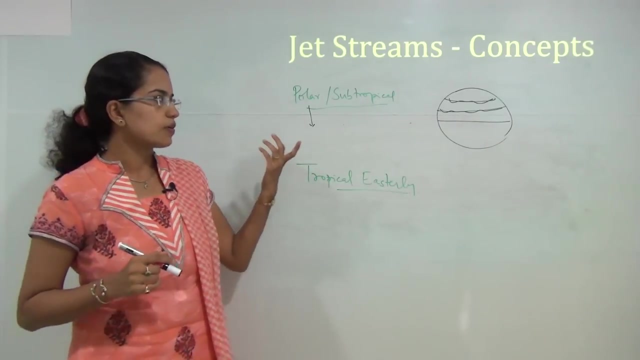 Now this is the polar jet stream jet stream and the polar jet stream that would run, respectively, in these regions. Now what is happening? as we have already talked about the concept of angular momentum here, when the air is being heated, the hot air moves up. 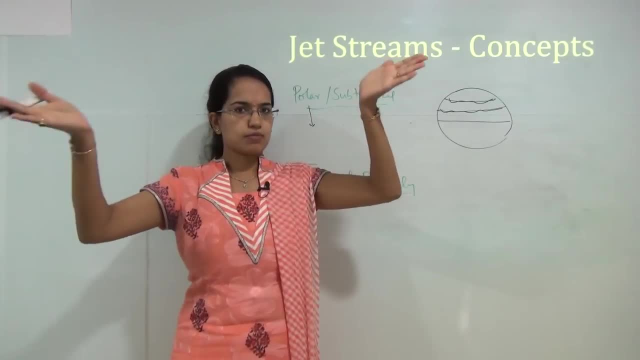 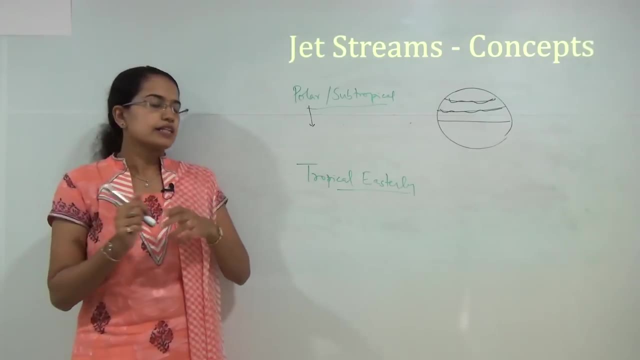 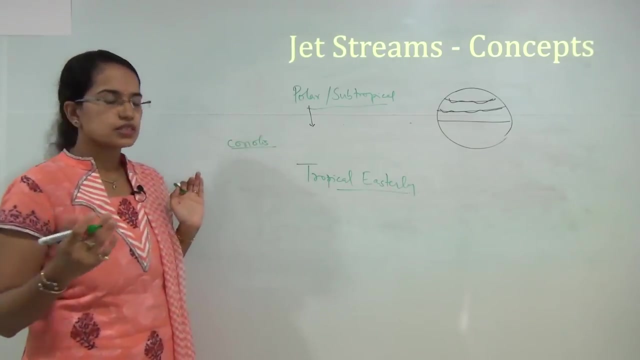 So hot air parcel is moving up and it diverges in the upper atmosphere, as we have talked about in the circulation system or the wind circulation patterns. Now again, what is important to know here is the impact of Coriolis force. So because of the Coriolis force in the north, it would move towards east. 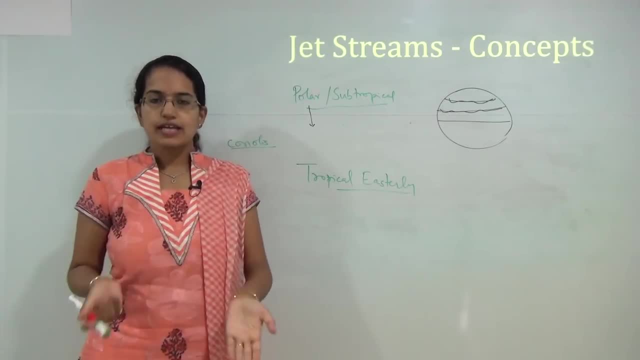 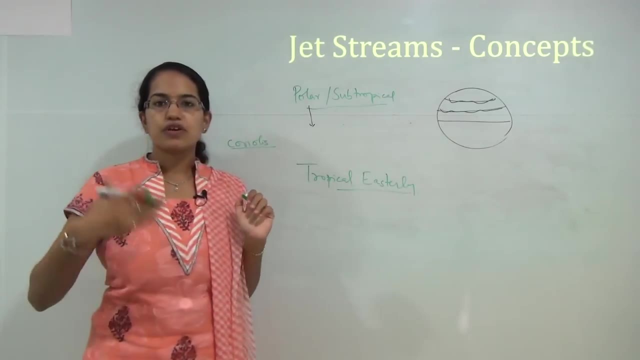 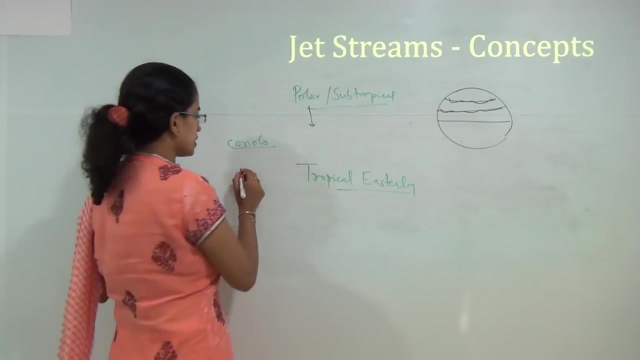 So, when it would move towards east, what would happen is so, as the air is moving northward, you have the curvature of the earth that is here. and since the air is moving northward, what would happen? the air would move close to the rotational axis, or the axis of rotation. 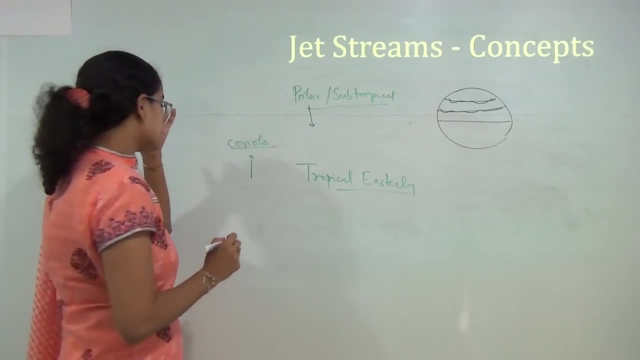 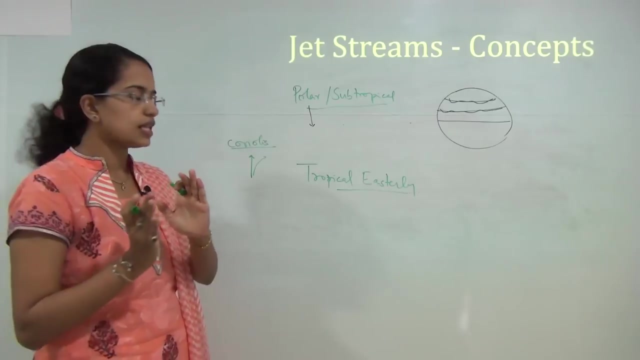 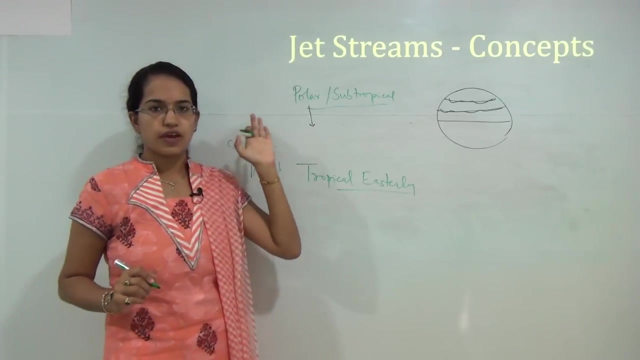 So you would have a northward movement, with the wind moving closer to the rotational axis And since it is moving closer to the rotational axis, it would decrease the radius. Now, once we have the radius that is decreased, based on the conservation of angular momentum, you would have the velocity of the wind would increase. 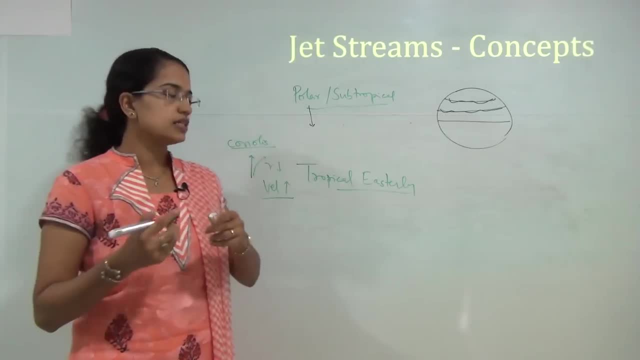 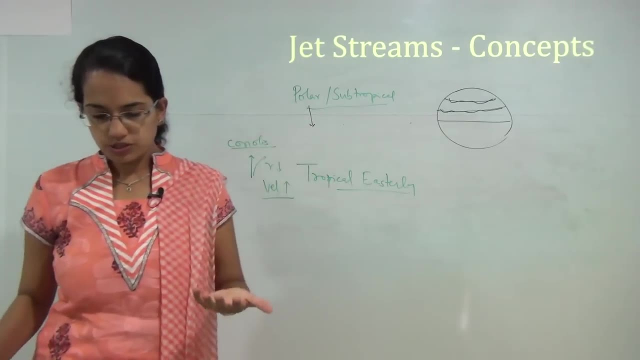 Now these strong winds are blowing east, but they are originating from the west, or an observer to an observer, it would look as a wind from the west, So they are also known as west winds or westerlies, But they are moving to the north. 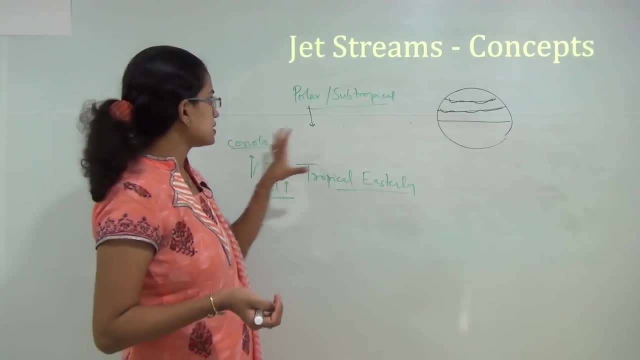 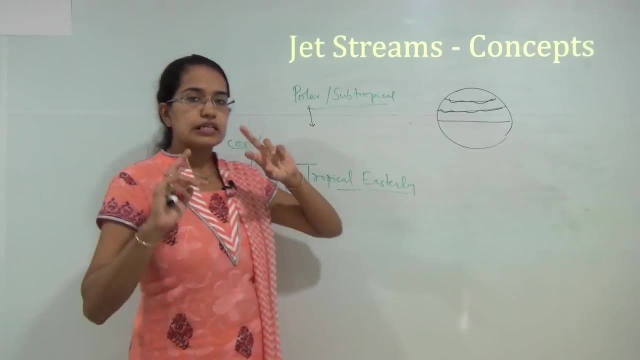 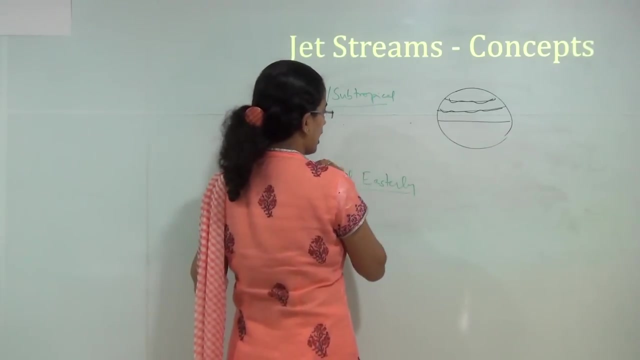 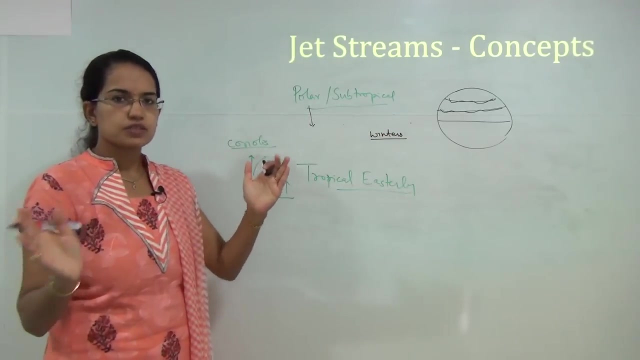 They are moving towards the eastern direction And so we can understand. this is how the polar jet streams are formed. Now again I can say increase in the temperature difference would make the winds much more stronger. So if I say you have during the winters, you would have much wider temperature difference. between the summers and the winters, or the extremes in the temperature, would be much higher. That means, since the temperature gradient is much higher, the polar westerlies that are created or the jet streams that are created in the winters would be much, much stronger as compared to the summer season. 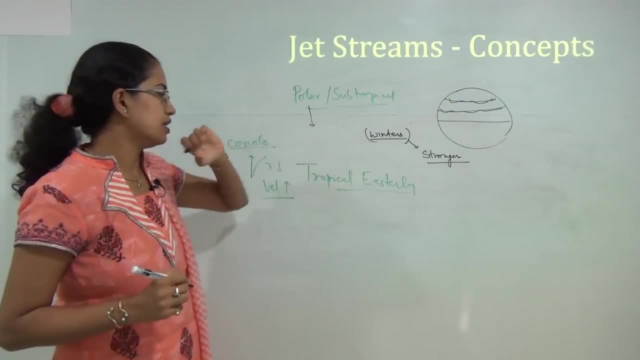 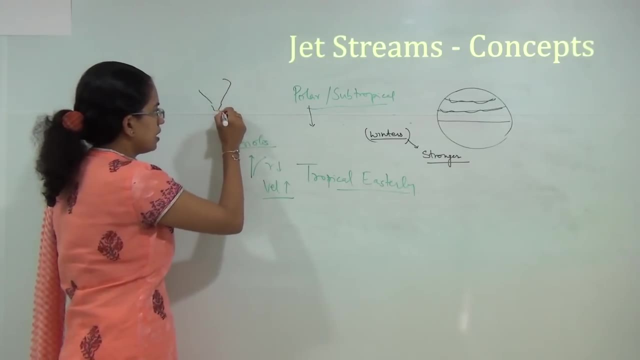 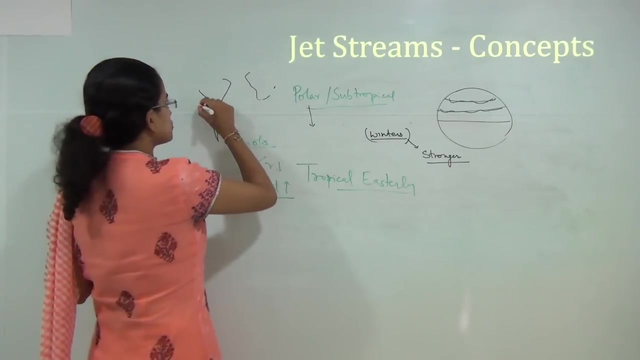 So that is one thing to note about the polar jet streams. Now again, you have, let's say, this is the map of North America, and you have South America here And you have the European region here. Now let's say if this is the actual polar jet stream that is running. However, because of the changes in the temperature gradient and pressure gradient, this polar jet stream might change its path in certain seasons. So this would be an alternate path for the polar jet stream. So, based on the temperature gradient and the pressure gradient, you have the polar jet stream. 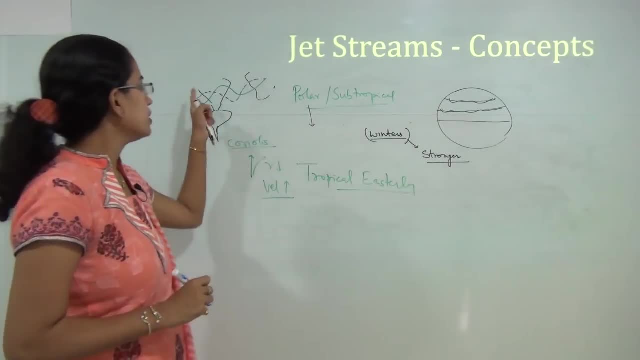 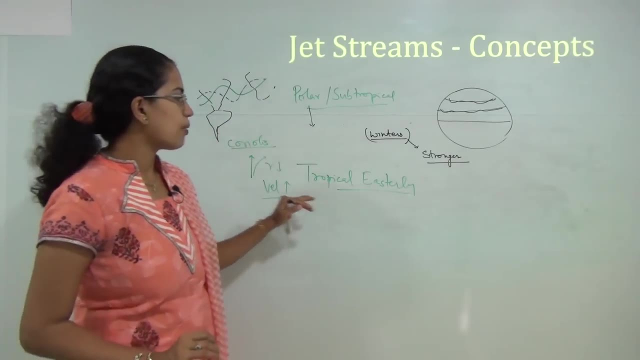 So this is the polar jet stream. So this is the polar jet stream. So this is the polar jet stream. Now, here you have the various path of the jet stream that could be seen in the atmosphere Now. formation of the tropical easterly jet stream. 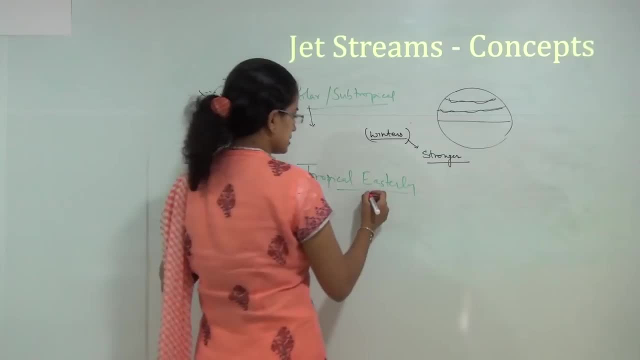 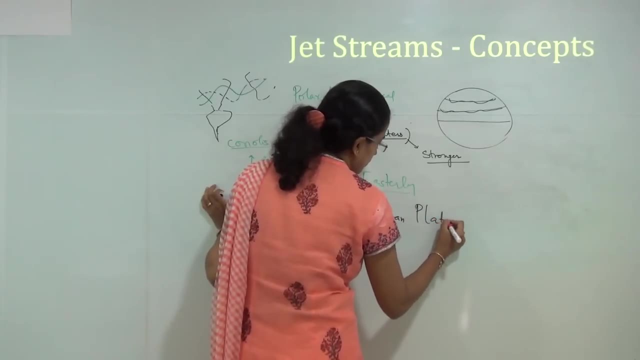 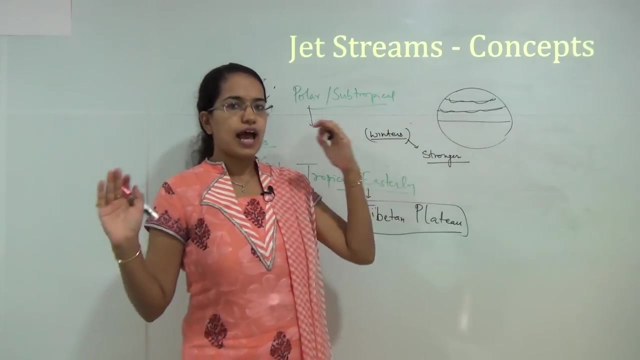 Now a typical case for formation of tropical jet stream is attributed to the Tibetan Plateau. We have already talked about Tibetan Plateau in a separate class. We will again refer it here because this, as we mentioned in the previous class, is a huge land mass. 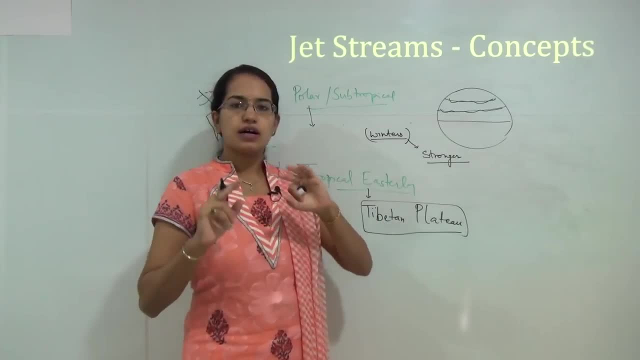 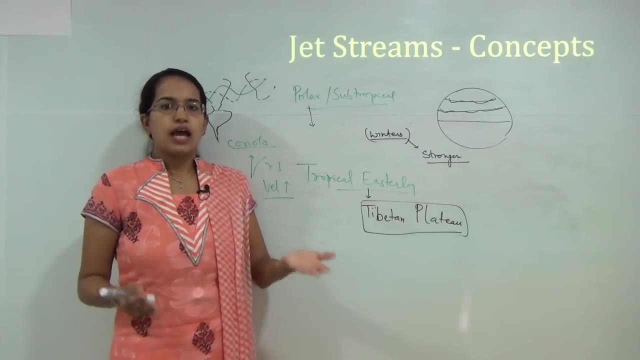 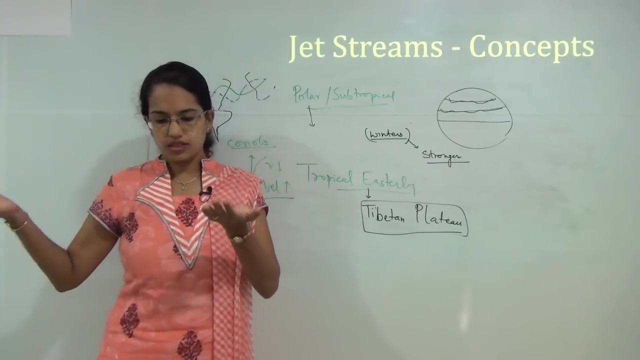 And that huge land mass at such a height affects the weather conditions. So this is the typical case. the equilibrium temperature affects the climate of the region. Now what happens is warming of the land takes place at the Tibetan plateau, and this warming that is taking place at the Tibetan plateau is much more as compared to the ocean, to the 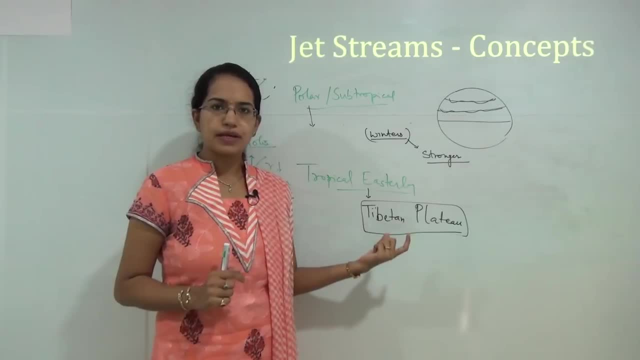 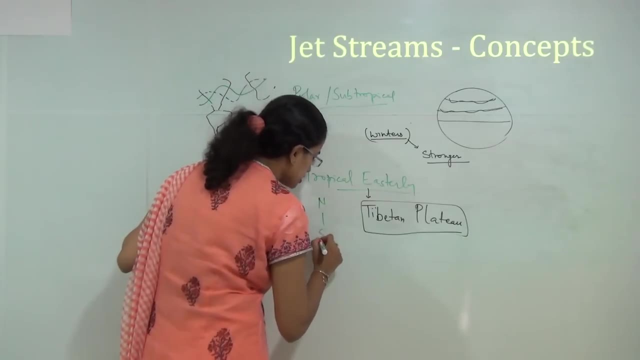 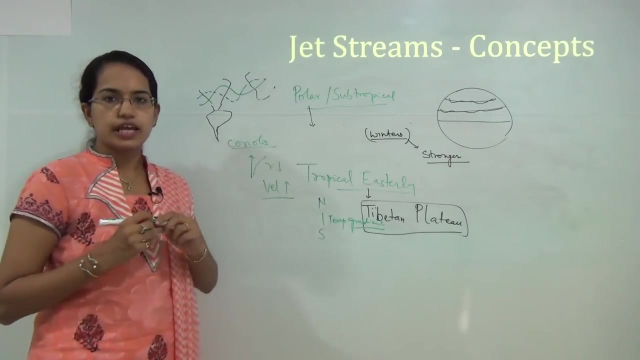 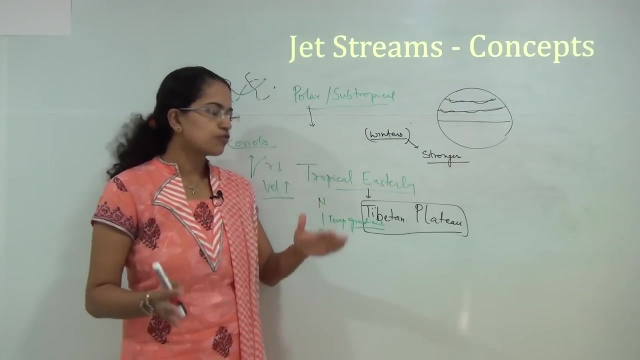 south of it. As a result, what would happen is there would be creation of a temperature gradient, and this temperature gradient would be north south temperature gradient. Now, this north south temperature gradient would again impact the winds that are originating, So air will flow towards south, to the south, from the Tibetan plateau. 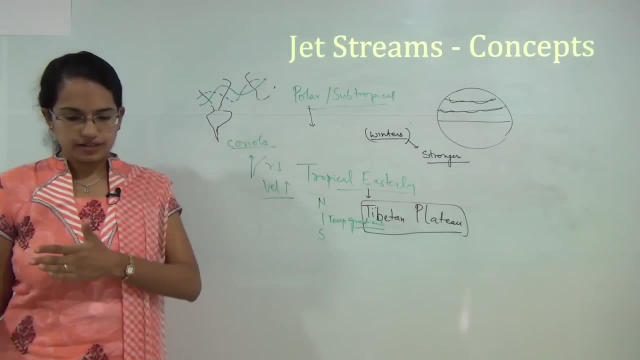 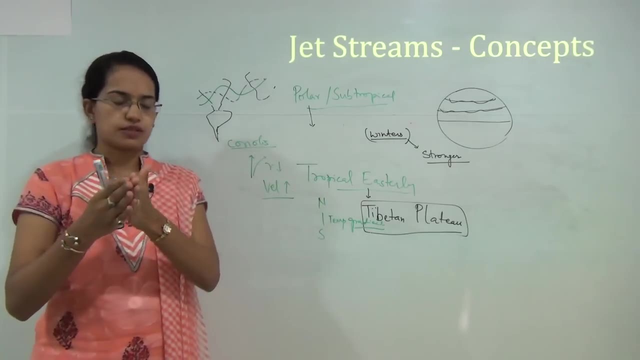 When it is flowing south, it would deflect the air and that, as it moves south, what would happen is it is moving away from the axis of rotation. So when it is moving, When it is moving down, it is moving southward, it is moving away from the axis of rotation. and since it is moving away from the axis of rotation, what would happen here is the radius would increase, and since there would be increase in the radius again, there would be decrease in the velocity, and these are attributed to the formation of the tropical easterlies. 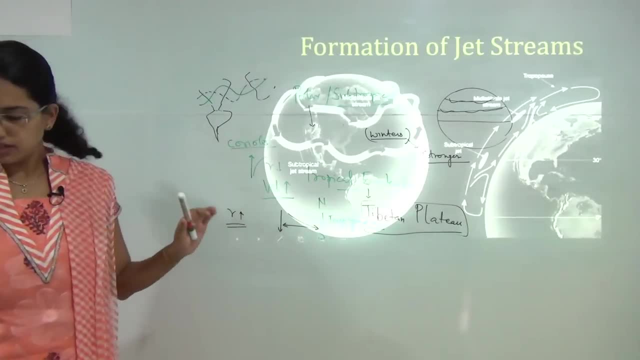 Now tropical easterlies in certain cases can be much more strong. Usually, tropical easterlies are not that intense as the polar jet streams are. Now we talked about the formation of the jet streams. so here you have the 3 cell diagram and you can see the regions where you have the jet stream formation. 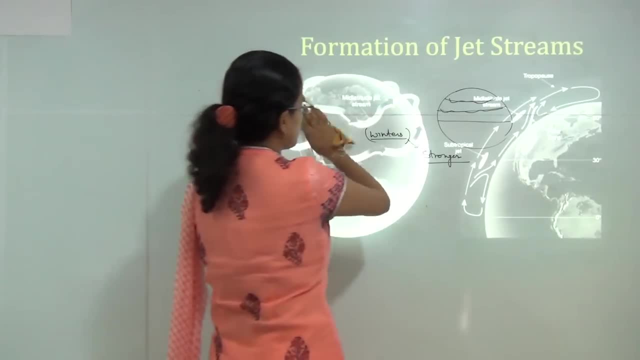 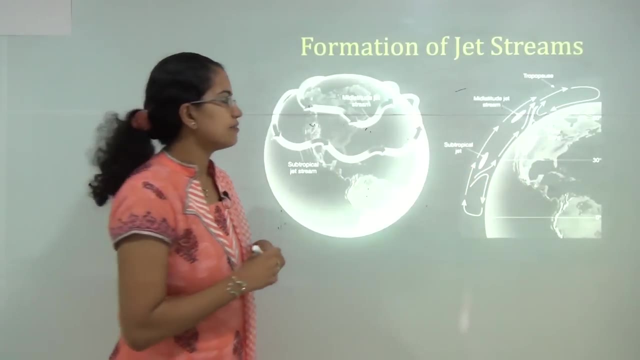 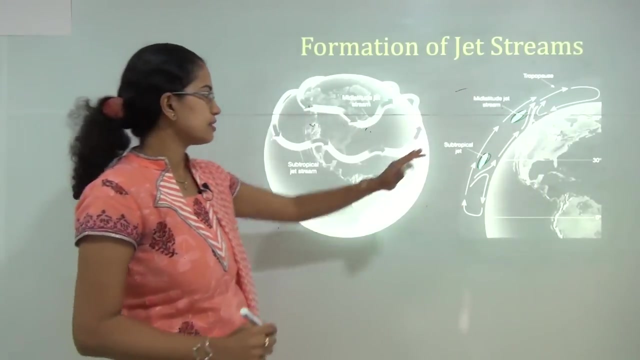 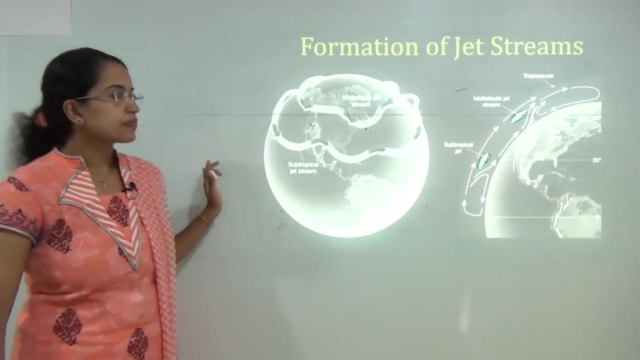 So you have the sub tropical jet stream formation and the mid latitude then, or the polar jet stream formation, and these occur in certain path and this path, as we said, is a meandering path. Now, when we talk about a mianderent particular formation, if you have the condition of the 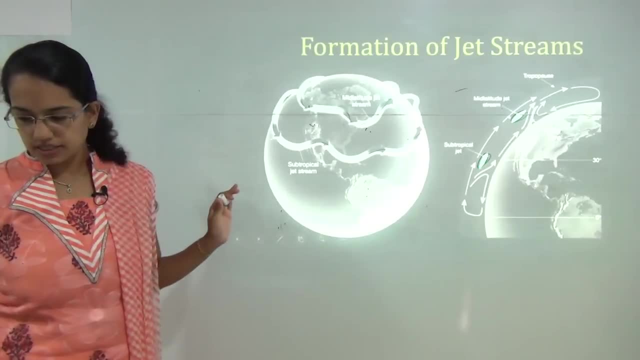 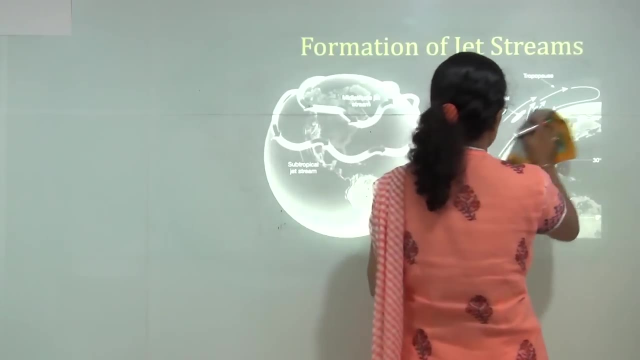 jet stream formation, then you know the present degree. you know it may be a bit different. then about the types of jet streams, we would classify jet streams into three basic types. since we have talked about the formation under three heads, we would again talk about the jet streams. 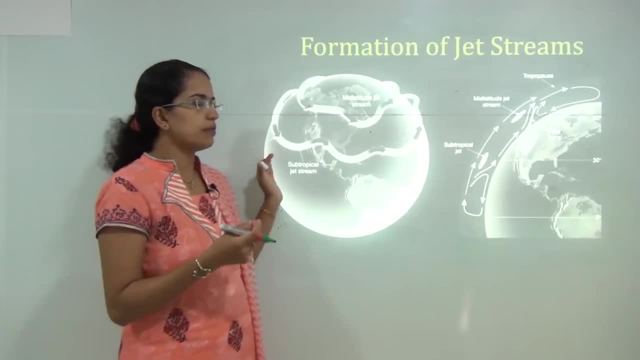 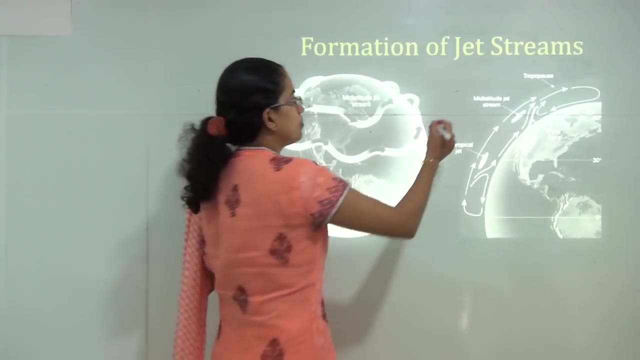 under three heads. So we will quickly go through the main points or the main highlights of each of the jet stream. So let us first talk about the mid latitude jet stream or the polar jet stream. So mid latitude jet stream is also known as the polar jet stream. 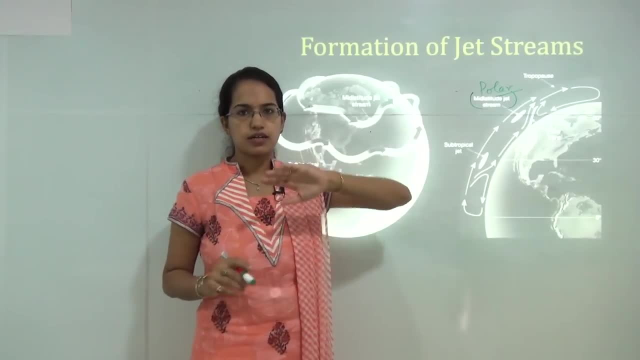 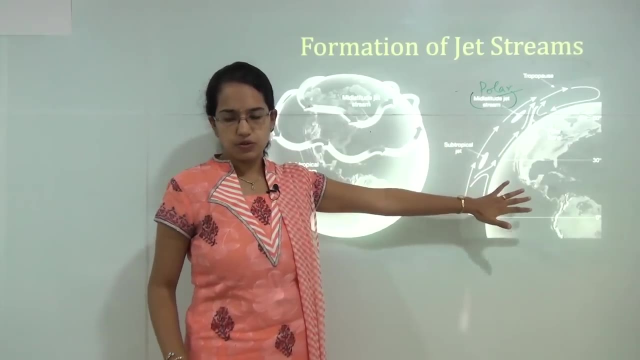 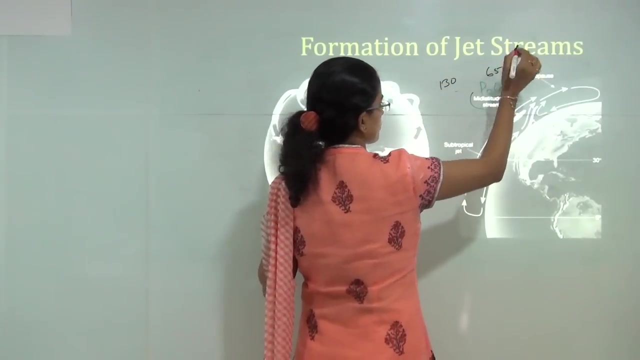 These are one of the most intense jet streams that occur on earth, usually found at a height of 10 kilometer. The velocity is much higher as compared to other jet streams. The extremes can be ranging from 130 kilometer per hour in winters to around 65 kilometers. 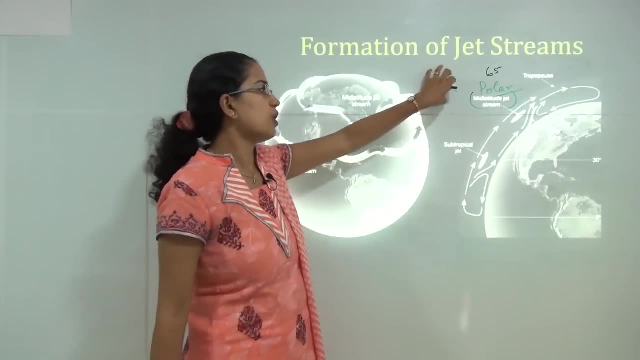 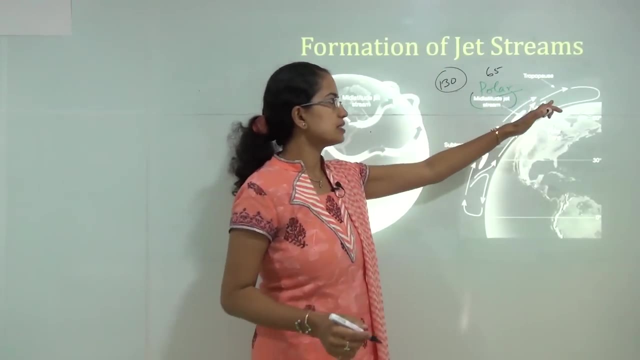 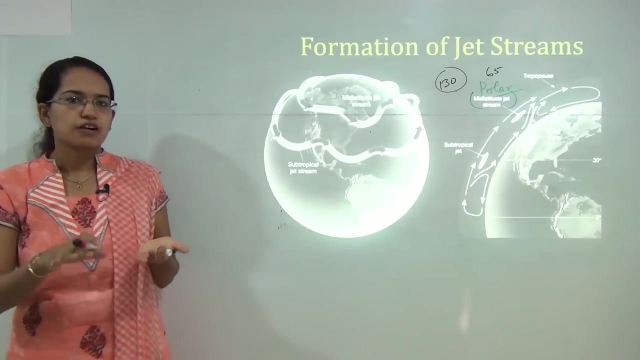 per hour. in summers- that means the winters- you have much more intense jet streams as compared to summers. Again, the reason remains the same: You have higher temperature contrast during the winters, and during the winters you have sudden cooling due to lack of the sun rays in the region. As a result, you have a sudden drop in the temperature and the differences in the temperature increase because of that. as we said, temperature and pressure gradient are the two major things that govern the intensity of the jet stream. So you have higher temperature difference as a result. the jet streams that would be. formed in this region would be much more intense. Okay Now, these polar jet streams are also formed due to the polar fronts that occur in this region, in the upper tropospheric level, where you have the formation of polar fronts and you would have the areas of divergence and convergence. 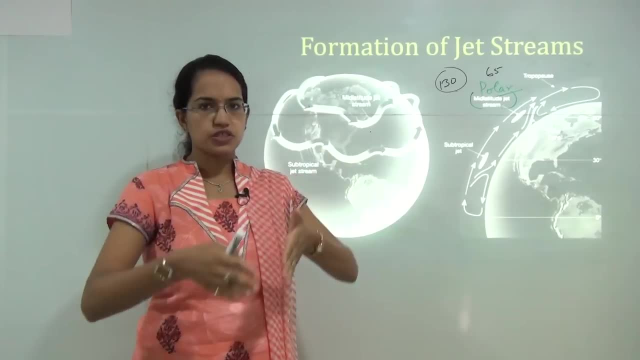 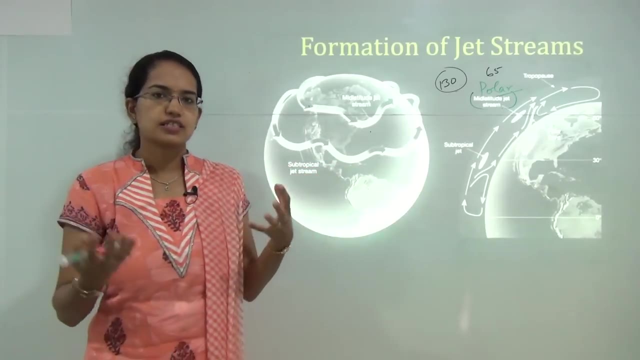 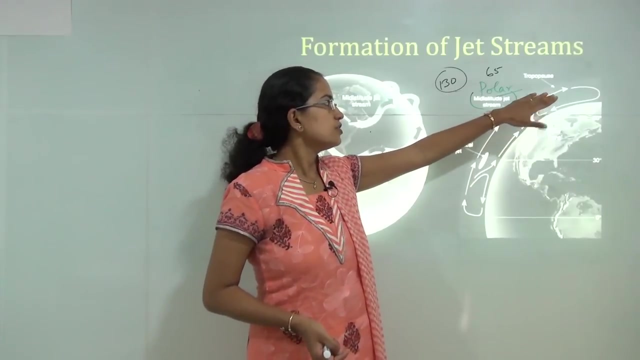 Now, the areas of divergence would be bringing the air downstream. However, you would have areas of convergence where you would have the cyclonic or the extra tropical cyclonic conditions that could be seen that we would refer under the head of cyclone in the later class. 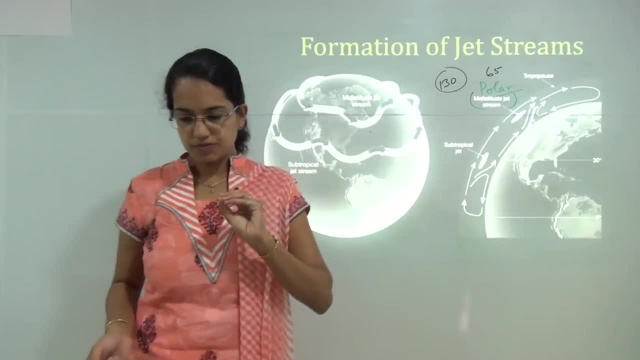 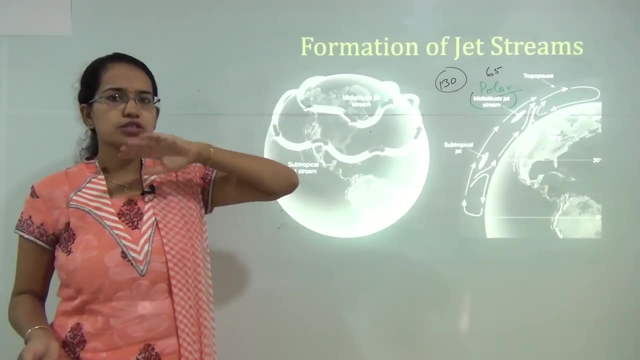 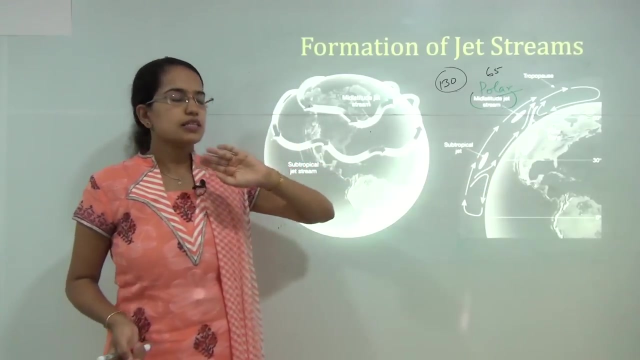 So these are the specific characteristics of polar jet streams. Now the next is the subtropical jet streams. Subtropical jet streams occurs around 13 kilometers above the subtropical high pressure area, Usually in the subtropical latitude they are found. These are less intense as compared to the polar jet streams. 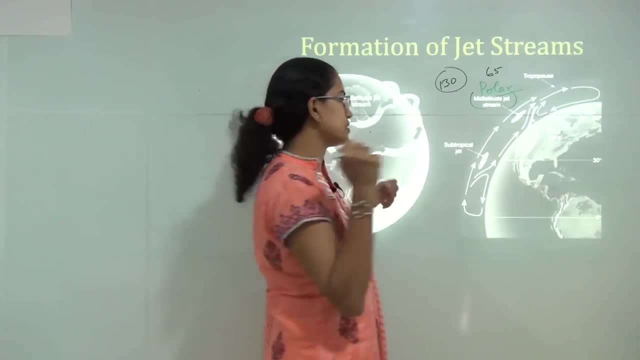 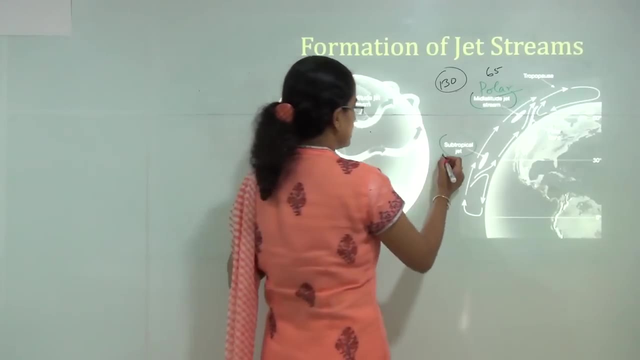 You have less temperature gradient and less pressure gradient. that can be seen in the subtropical jet streams. Okay, So again, they are intense only during the months of winters and early spring, because during winters and early spring you would have higher contrast in temperature. So, as a result, the jet streams would be much stronger or much intense during the winters and the early springs. However, in Asia, the tropical jet stream, which is also known as the westerly jet stream, is replaced by the tropical easterly jet stream. 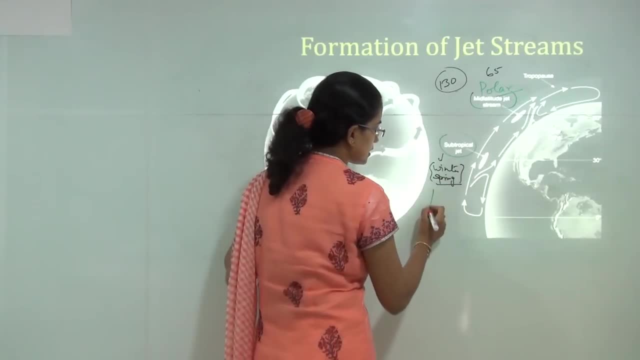 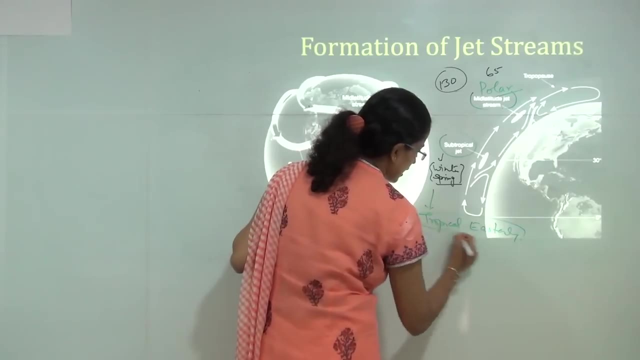 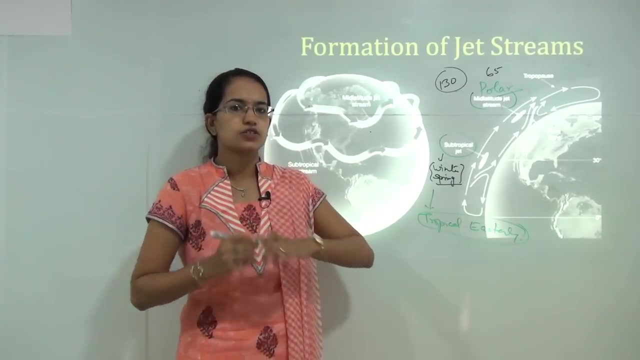 So this subtropical westerly jet stream is replaced by the subtropical westerly jet stream, Okay, by the tropical easterly jet stream in the parts of Asia, And that is again attributed to the presence of Tibetan plateau. You would have the tropical easterly, which occurs at the level of tropopause around 15. degrees north latitude, you would see the tropical easterly formation. It intensifies as you move towards the west of the south tip of India And because of the tropical easterly you would have monsoon conditions in India and parts of Africa. So you would have tropical easterly, which would attribute to the western African monsoon. 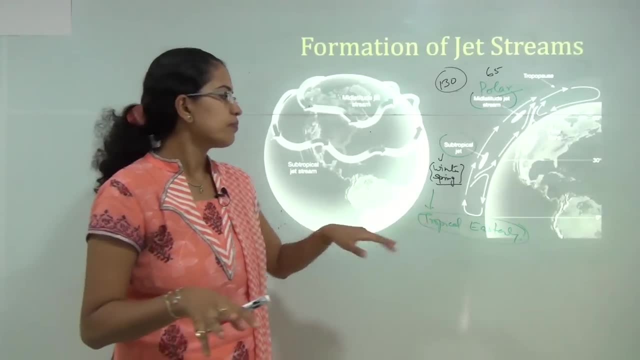 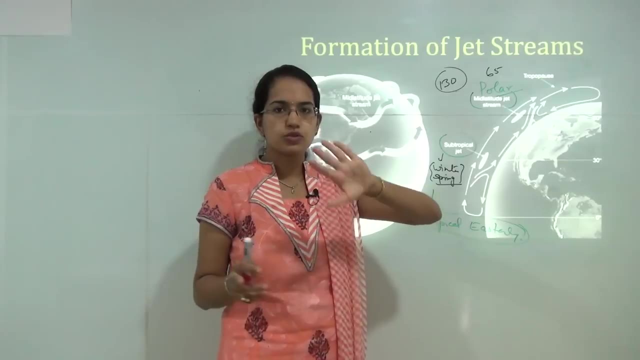 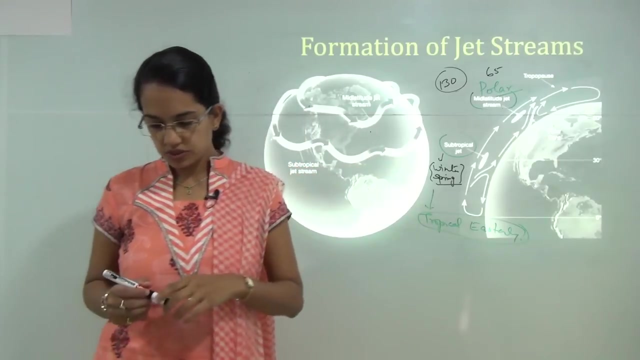 conditions. We have talked about the regimes of monsoon and there we have explained that the various regimes of monsoons. under that you have the African monsoon, which is divided into the west African and the southern African. So that would be responsible for the west African monsoon conditions.